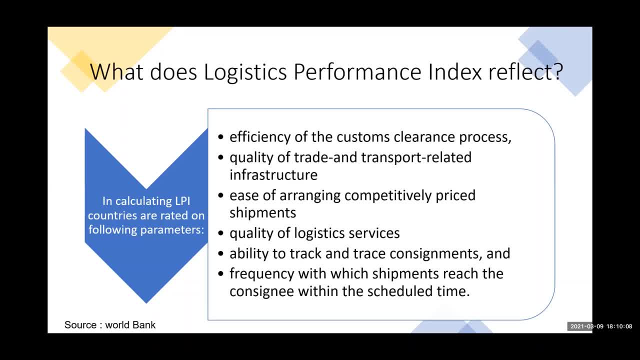 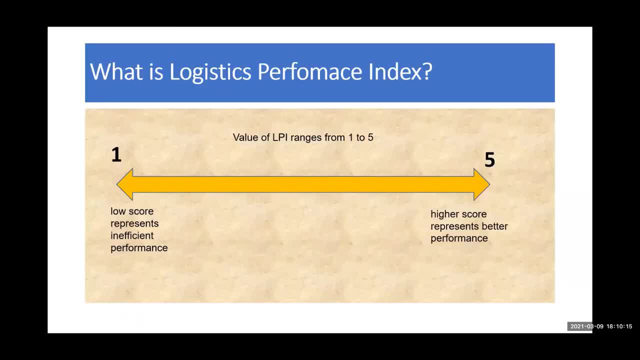 quality of logistic services, ability to track and trace consignment and frequency with which shipment reaches the consignee within the scheduled time. The value of logistic performance index ranges between 1 to 5, wherein a low score represents inefficient performance and a high score represents better performance. 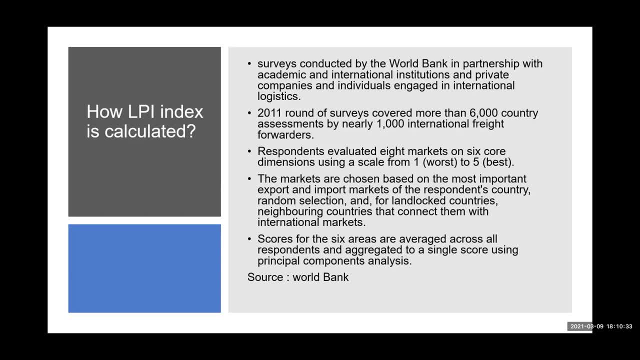 The LPI index is calculated by surveys conducted by World Bank in partnership with academic and international institutions and private companies and individuals engaged in international logistics. The 2011 round of surveys covered more than 6,000 countries' assessments by nearly 1,000 international freight forwarders. 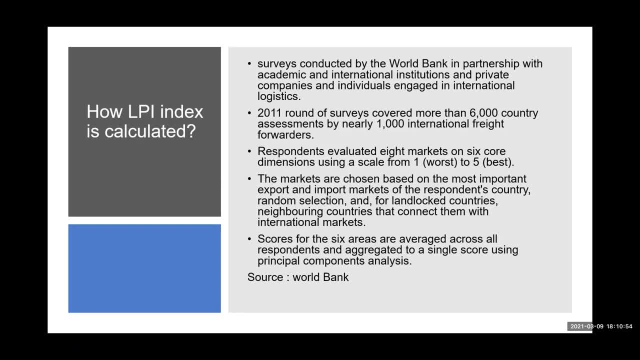 Respondents evaluated 8 markets on 6 core dimensions, using a scale from 1 to 5.. The markets are chosen based on the most important export and import markets of the respondent country and the most important export and import markets of the respondent country. 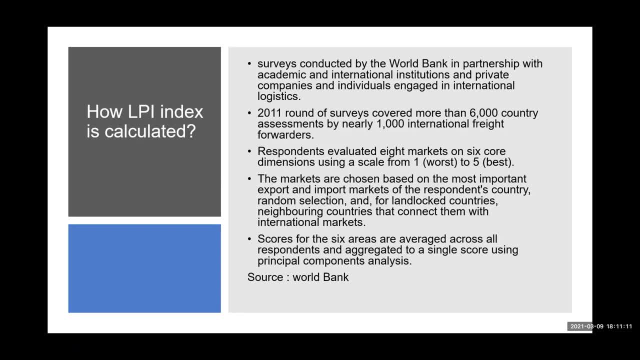 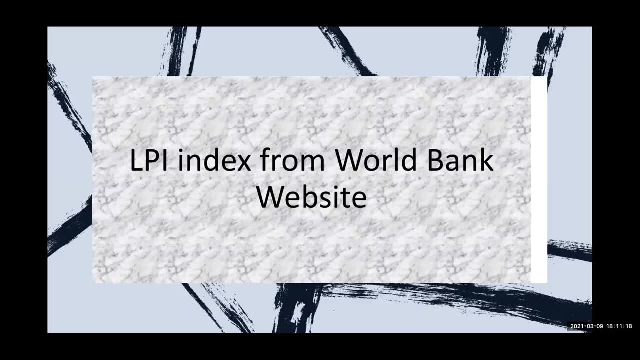 The scores for the 6 areas are averaged across all respondents and aggregated to a single score using principal component analysis. We will also learn how to extract the LPI index from the World Bank website. For this, you have to log on to the World Bank website, which is: 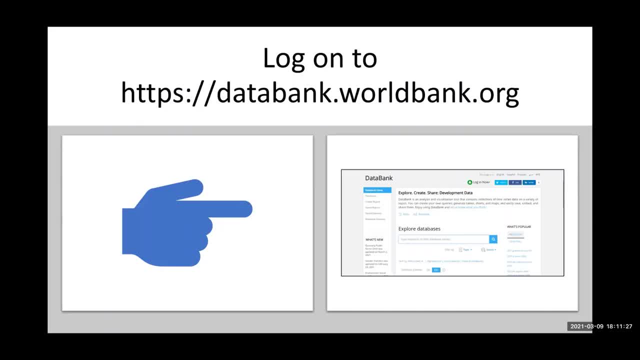 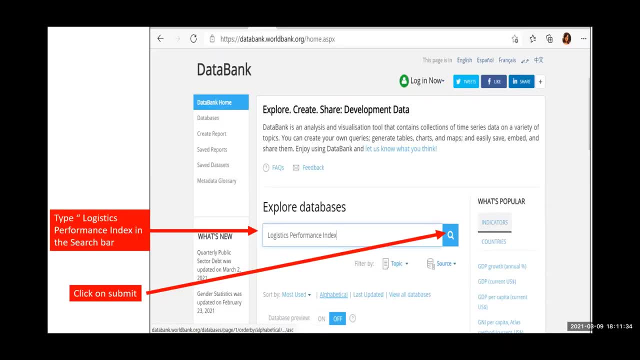 databankworldbankorg, You will also learn how to extract the LPI index from the World Bank website. So for this you have to log on to the World Bank website, which is databankworldbankorg. This will be the home page when you will log on to the website and you have to type. 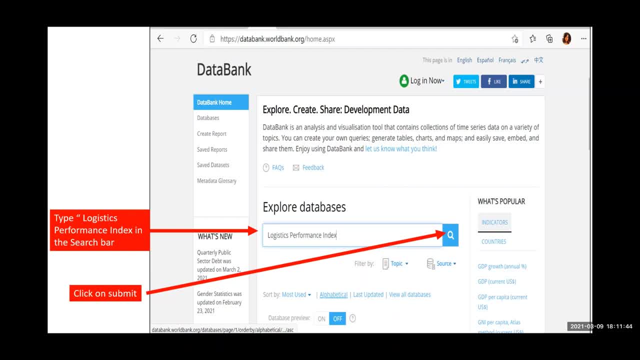 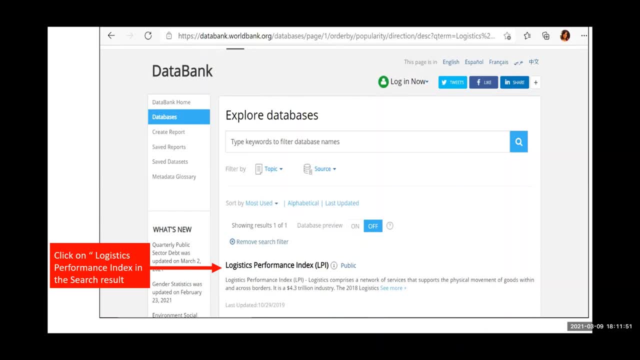 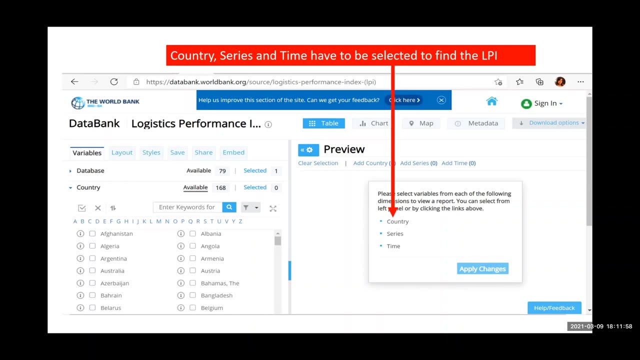 logistic performance index in the search bar and click on the search option- summit option- In the search result, logistic performance index will be visible. You have to click on that and you will be routed to the next screen wherein you have to select the parameters, like country series and time to find out. 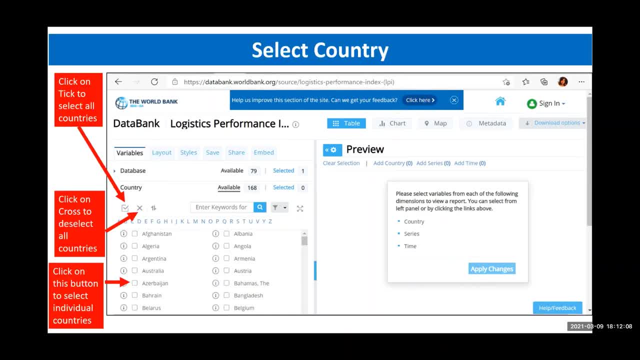 that you are in a country with logistic performance index. Let's see how to identify the tit button. For this you have to juicy the country sign in box and select lang to the country son field To choose a country. you have to click ok to enter what country you want. To select each country, just click on the tick. 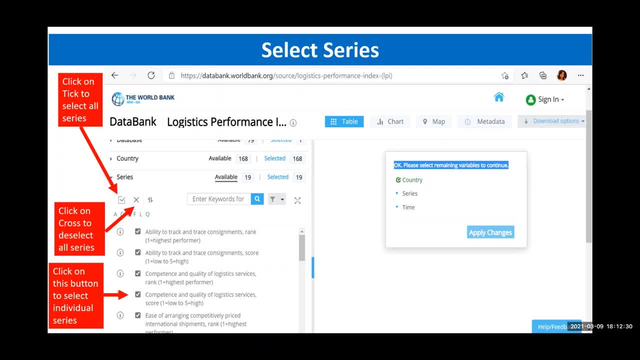 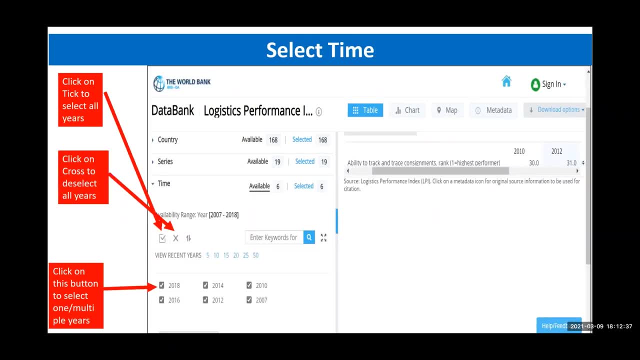 button to select all the country and click cross. go to to selectретite all camps. Ils select individual series. Same thing for time. you can click either on the tick or the cross or the individual buttons, So you can select either all the six years which are visible or 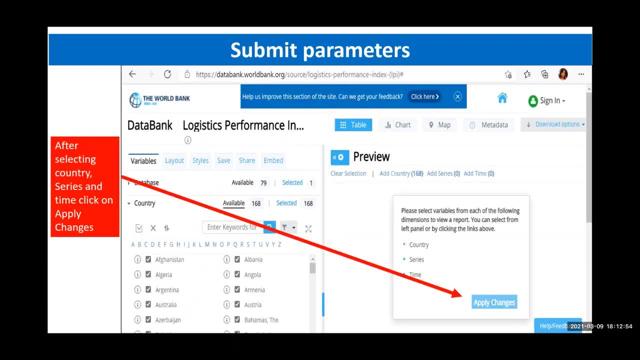 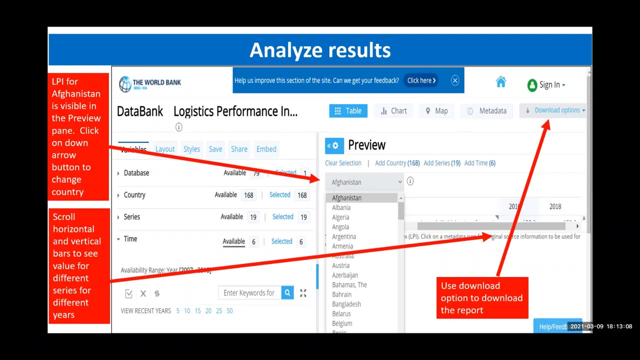 you can select one or two years as per your requirement. After you have selected indicators for country series and time, you have to click on the apply changes button to get the results. Results will be available in the preview option By default, since we have selected all the countries. 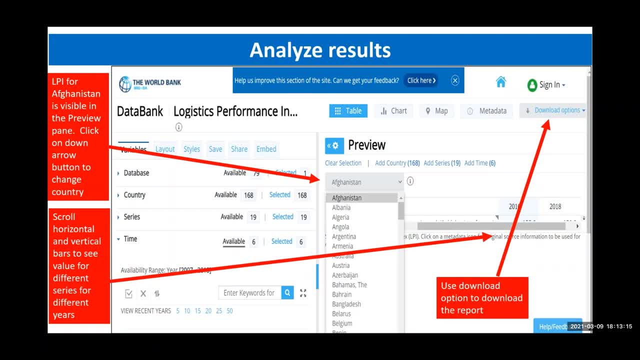 the LPI for Afghanistan is displayed first. If you want to see the LPI for different countries, you can click on the down button and you can select the countries from the drop down menu. You can now scroll the horizontal and the vertical bars to see the LPI index for Afghanistan. 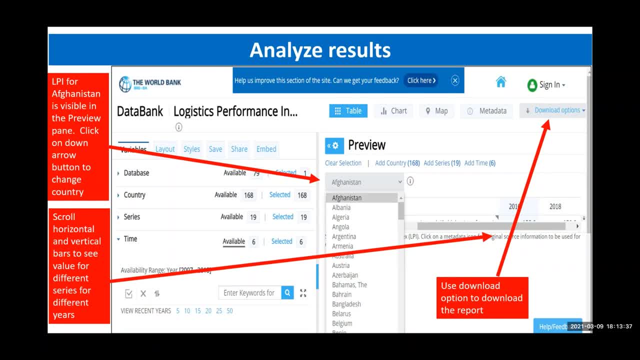 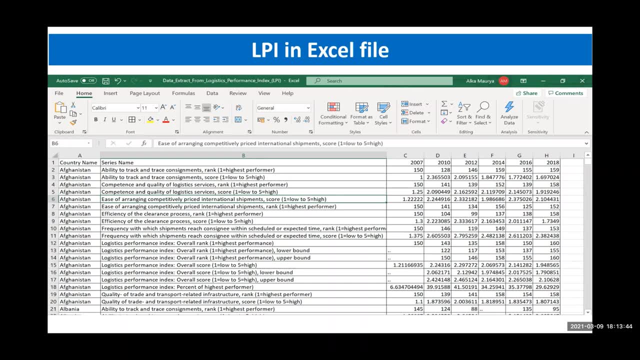 There is an option also to download the report. The report in the excel format looks like this. In this case you can see the LPI for Afghanistan and also for Albania. The second row indicates the ability of Afghanistan to track and trace consignment. The country ranked 159 in 2018.. 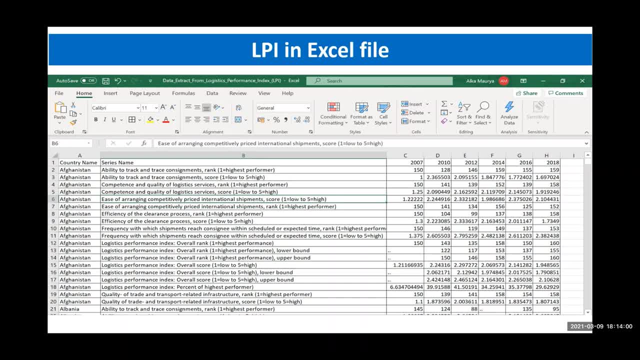 The scale of the google report is 1 to 5 and it ranks 1.69.. Similarly, for the competency and quality of logistics services, its rank is 158 out of 60 and its LPI index is 1.9.. So, for all the 6 parameters, 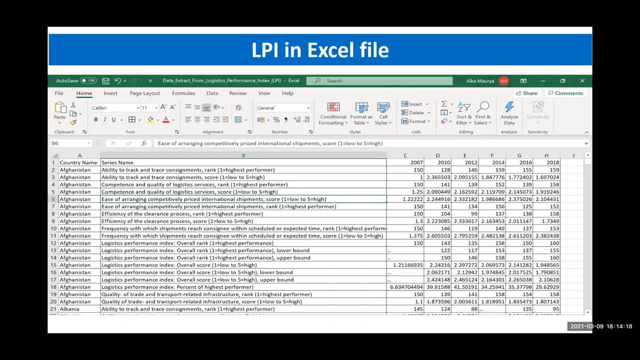 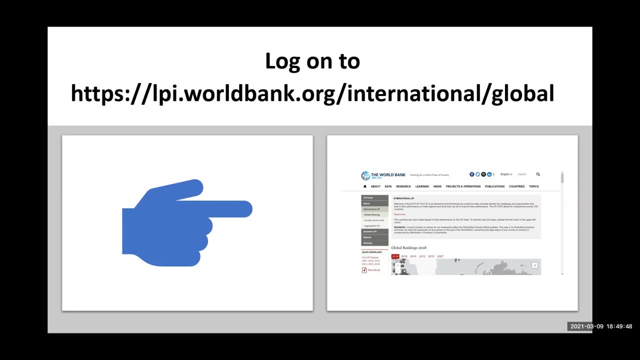 you can see the rank of the country and the LPI index. Similarly, when you download the report, in this file, I have LPI index for all the 160 countries. Alternately, you can also log on to the World Bank website, lpiworldbankorg. slash international, slash global.